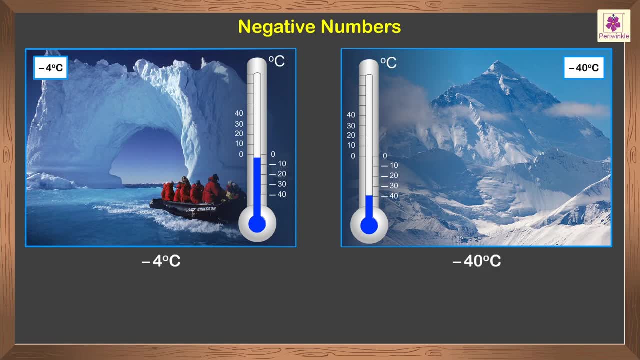 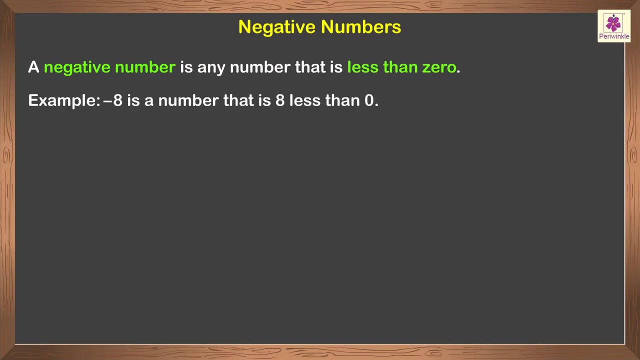 4 degrees Celsius or even below negative 40 degrees Celsius. The numbers negative 4 and negative 40 are less than zero and are called negative numbers. A negative number is any number that is less than zero. For example, negative 8 is a number that is 8 less than zero. 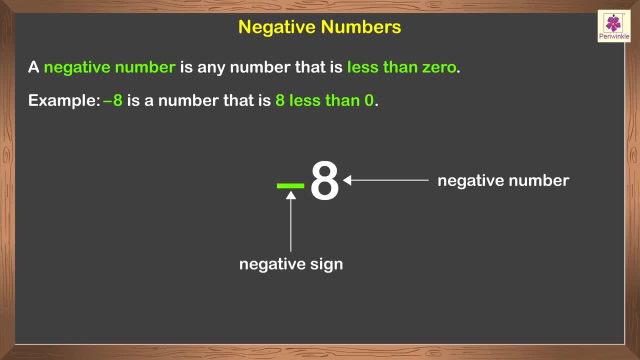 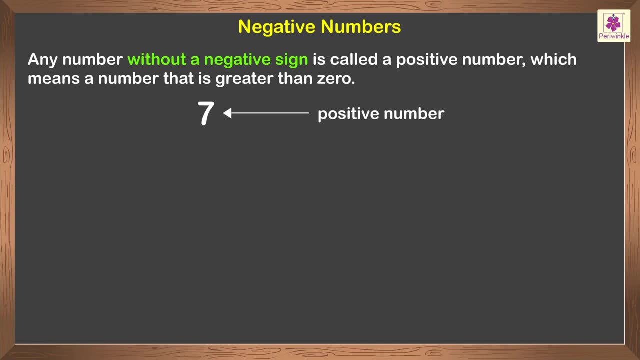 A negative number is represented with a negative sign. Any number without a negative sign is called a positive number, which means a number that is greater than zero. So, while negative 8 is negative, 8, 7 is positive, 7 or simply 7.. 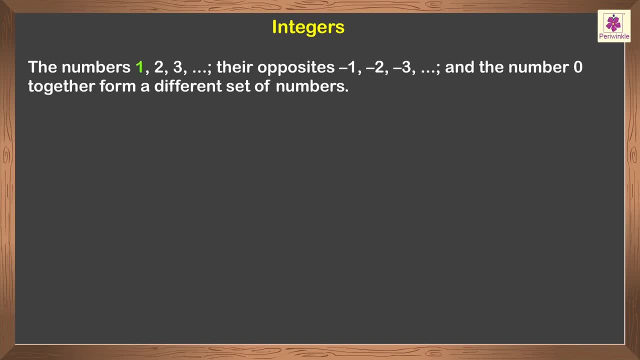 Integers: The numbers 1,, 2,, 3 and so on. they're opposites: Negative, 1. Negative 2. Negative 3 and so on, and the number zero together form a different set of numbers. Let us understand the set of integers with the help of the following diagram. 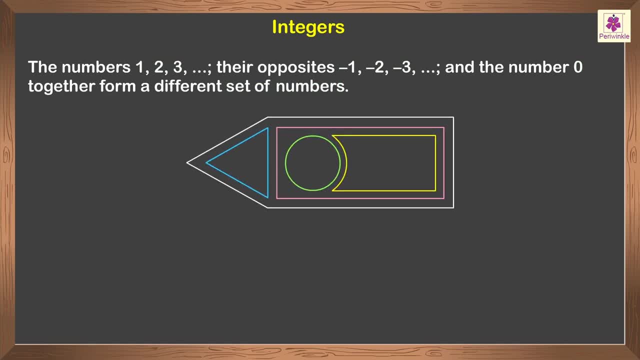 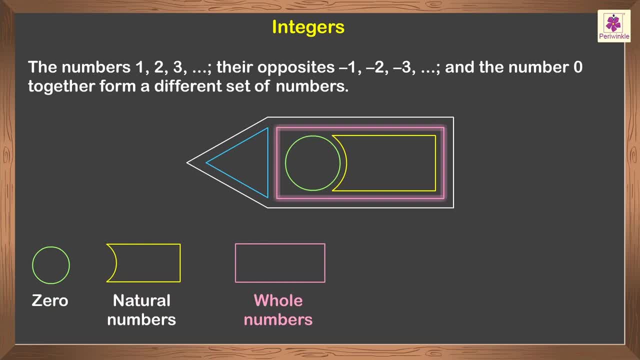 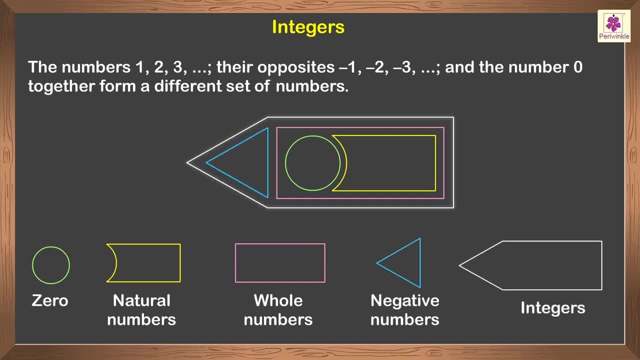 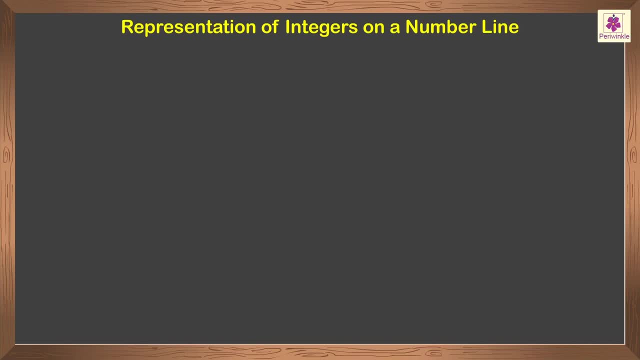 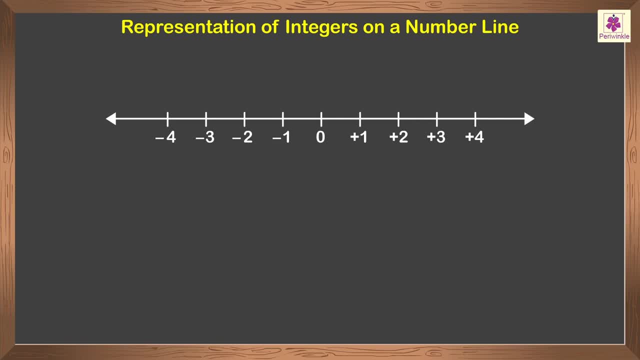 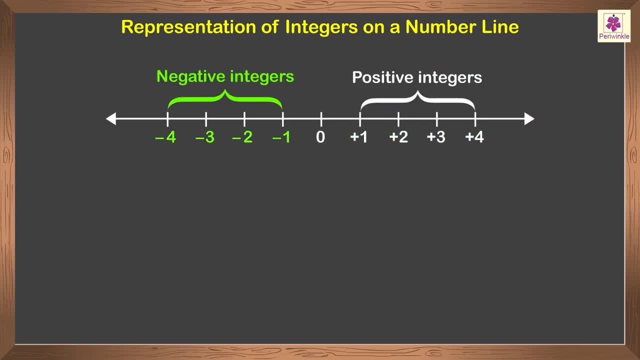 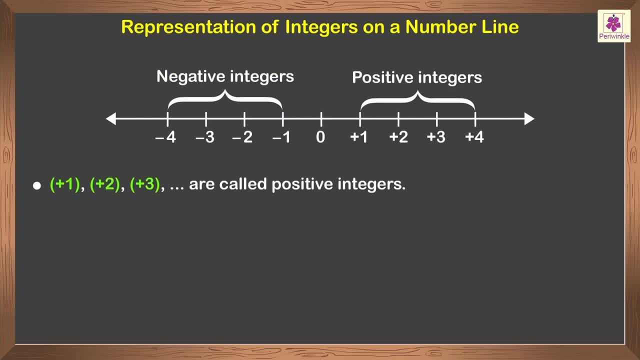 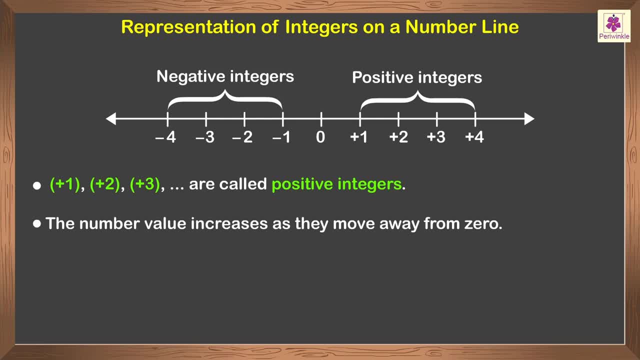 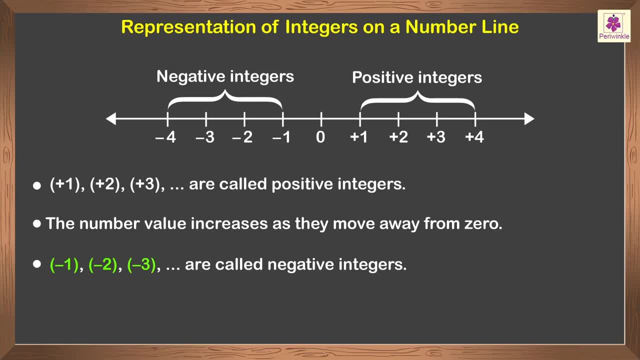 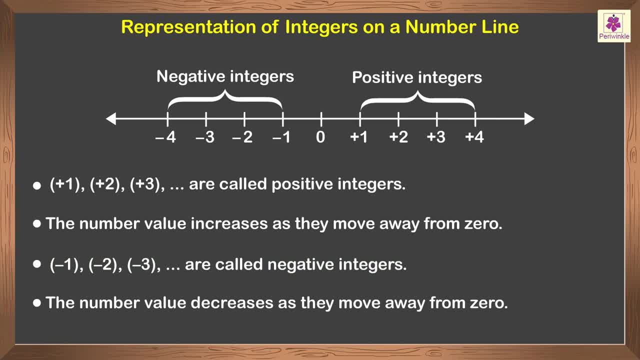 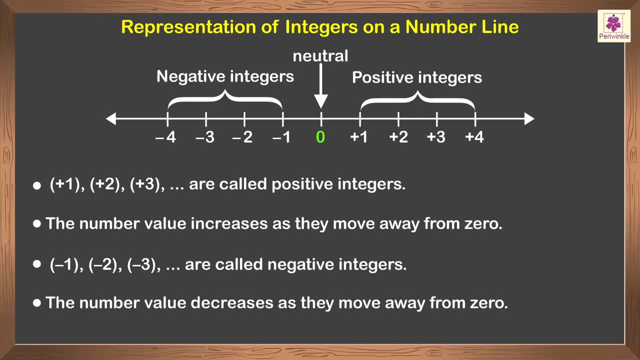 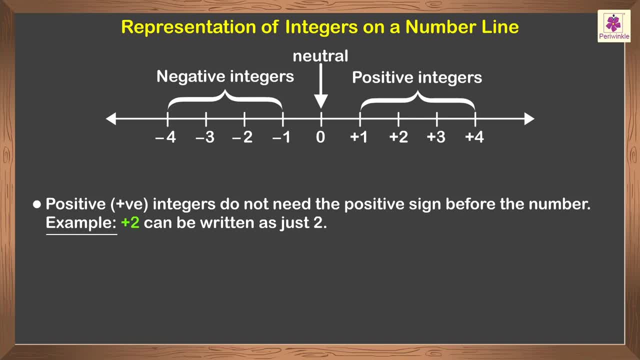 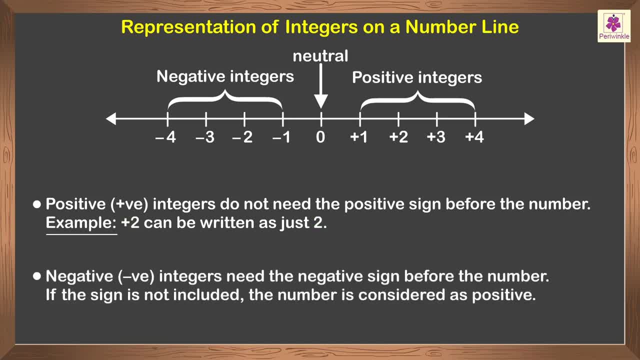 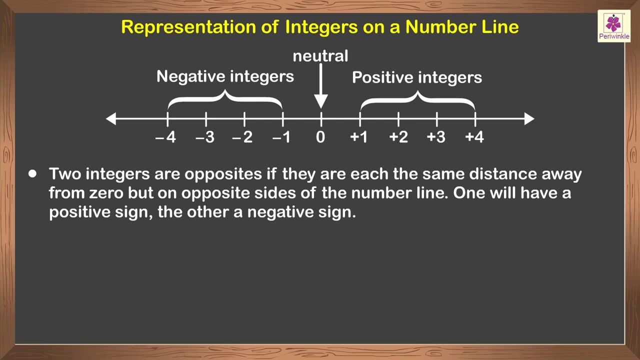 The triangle represents a number. The triangle represents a number. The triangle represents a number before the number. If the sign is not included, the number is considered as positive. Two integers are opposites if they are each the same distance away from zero, but on opposite sides. 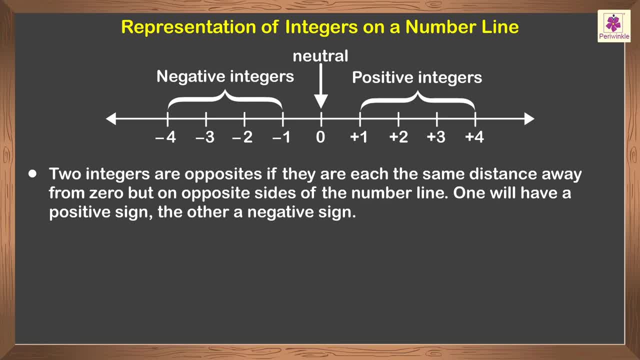 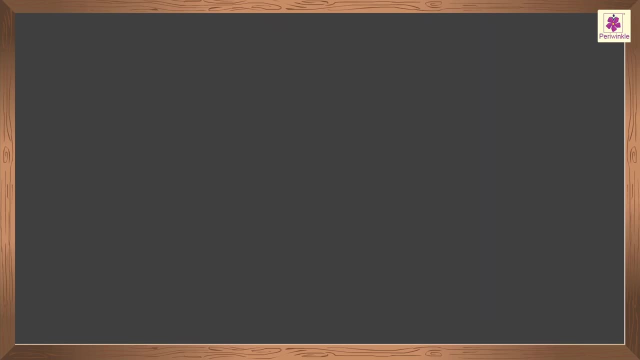 of the number line. One will have a positive sign, the other a negative sign. In the number line shown here, positive 3 and negative 3 are opposite numbers. Now let us look at different situations where we mark a number either as positive or negative.